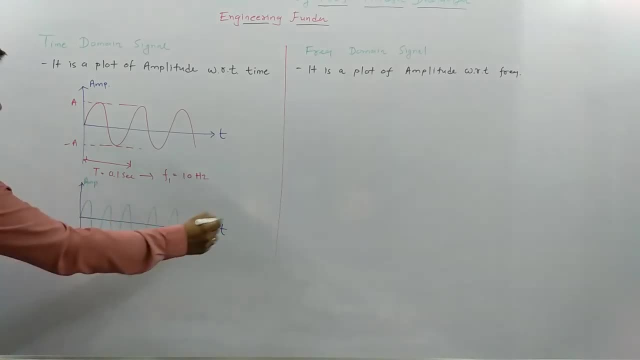 time, And if I say time period, that is 0.05 second. So based on that we can identify frequency F2.. That is 1 divided by 0.05.. So that will be 20 hertz. 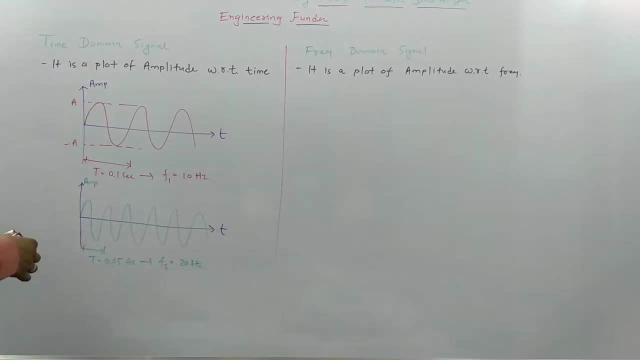 Now again, if I merge these two signals, so in that case we will be finding resultant signal is very complex. So first signal that we have plotted already, ranging in between plus A to minus A, like this. So here this is first signal and that is ranging by plus A to minus A. Second signal that is: 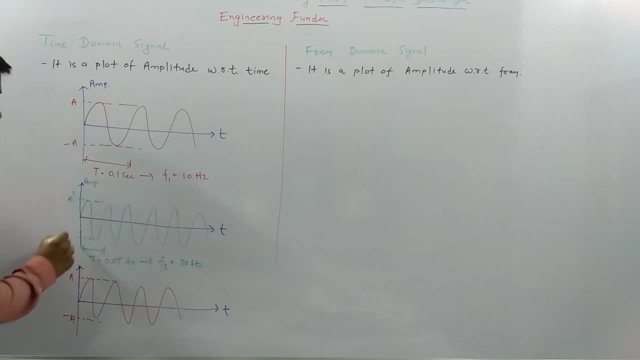 let us say it is ranging in between plus A' to minus A' and its frequency is 20 Hz. So that signal will be somewhat this, Where its amplitude, that is, ranging from plus A' to minus A' See, that is how that signal will appear. 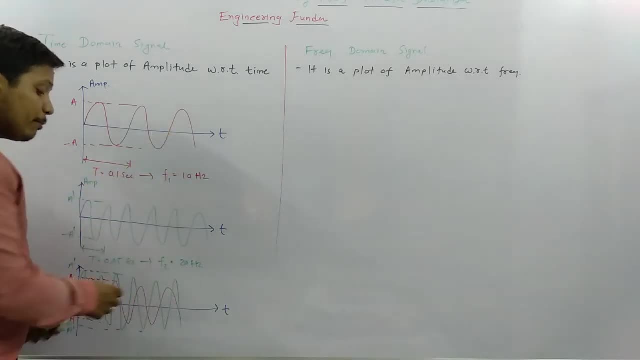 Now, if you see this resultant signal of these two signals, that is very complex. This signal of these two signals is very complex. So when we see time domain analysis By time domain representation of signal, you will be finding signals are very complex. This is just a case of two signal. 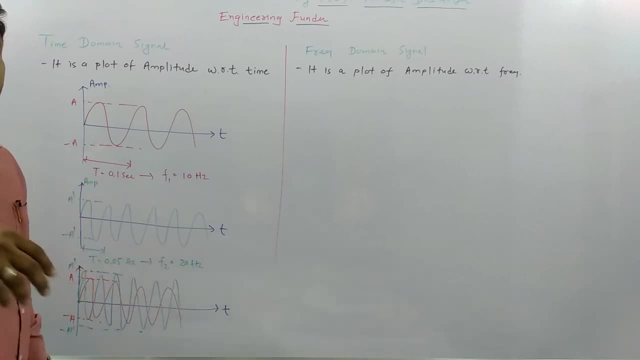 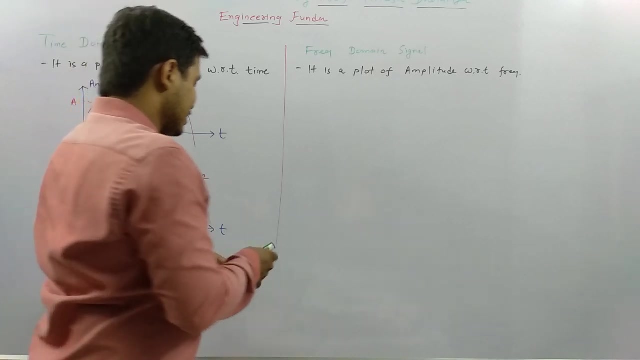 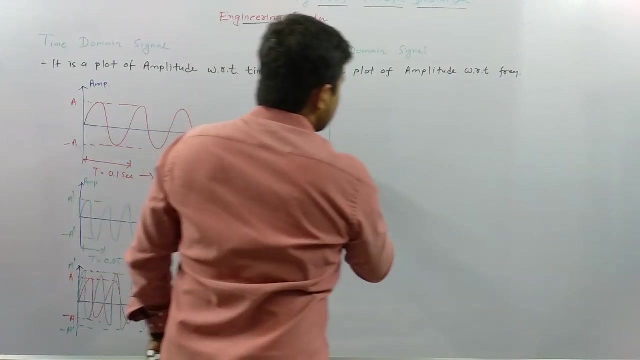 But if you consider 4 to 5 signal then you can imagine like how many, how much complexity that is there in signal representation. So to solve that problem we have frequency domain analysis. Now in frequency domain analysis We have A plot of amplitude with respect to frequency. 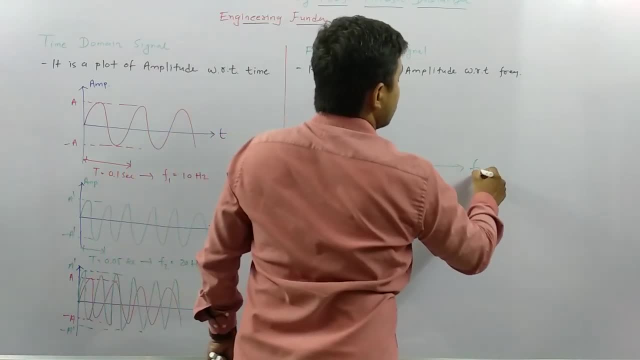 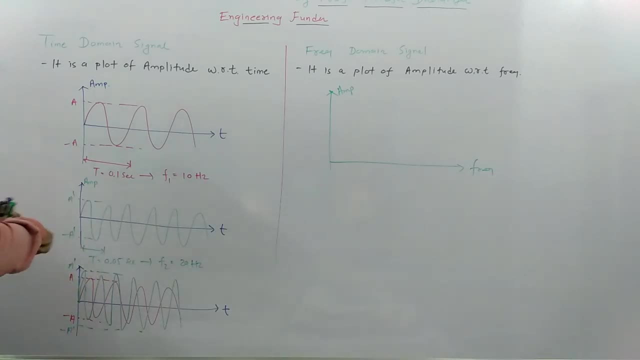 So we will be having amplitude with respect to frequency in frequency domain analysis. Now, if you see first signal, so that is having frequency 10 Hz and amplitude ranges by plus A to minus A. So when you plot that in frequency domain you will be finding its frequency is 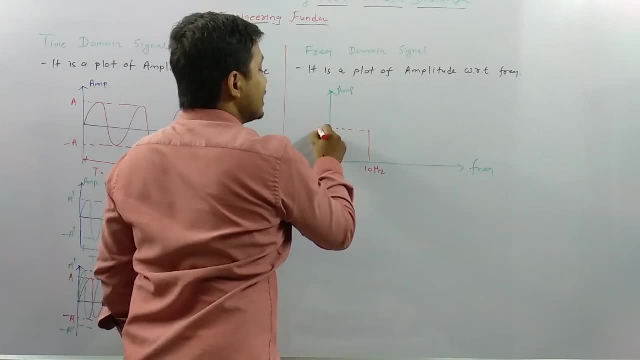 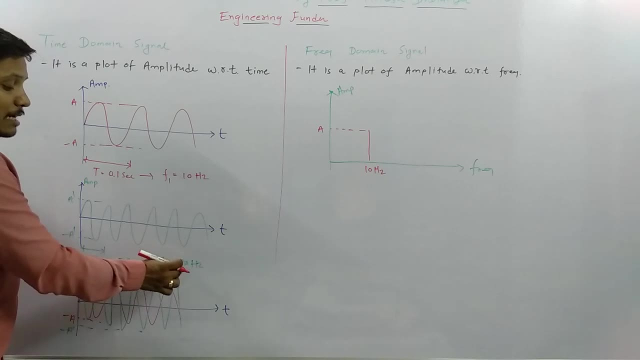 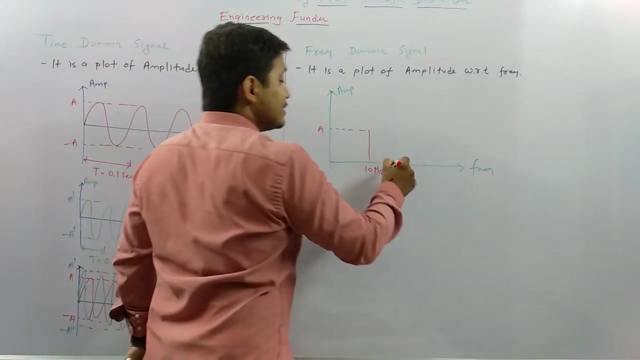 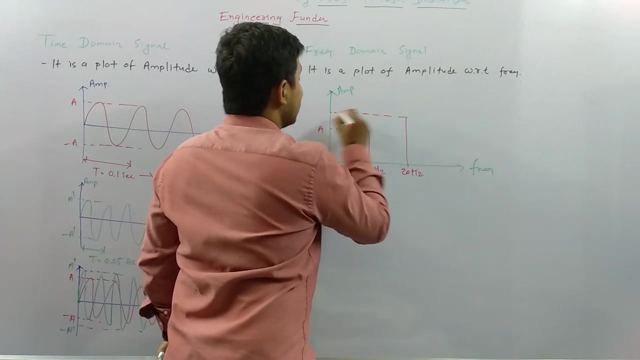 10 Hz And its amplitude that is A. And for second signal you have seen that frequency is 20 Hz and amplitude is plus A' to minus A' So here that second signal is having frequency 20 Hz, amplitude is A' So this is how simply we can represent that in frequency domain. 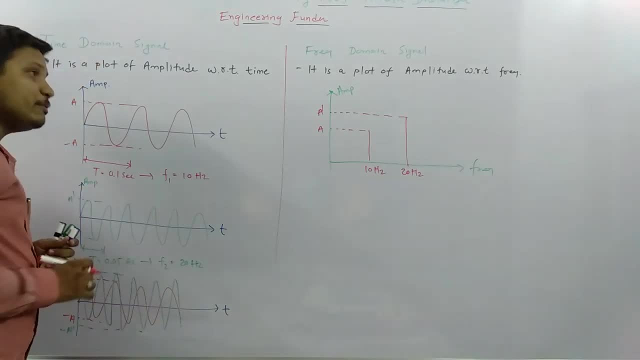 So this is how simply we can represent that in frequency domain. Well, it was so complex in time domain. So if multiple signals are there, complexity is more in representation of time domain signal, while that complexity is very less in frequency domain representation. So this is how the first few basic advantages which is there with frequency domain. 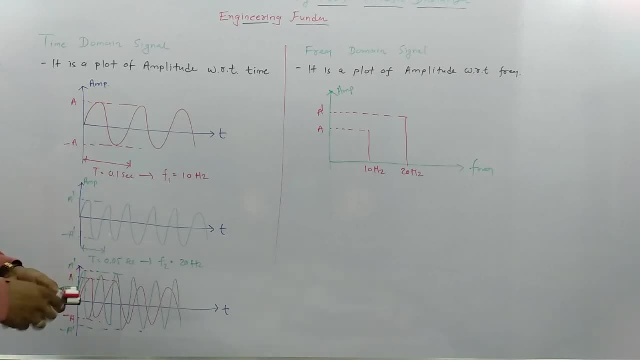 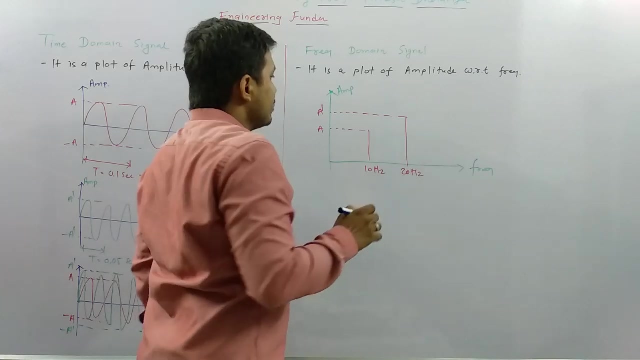 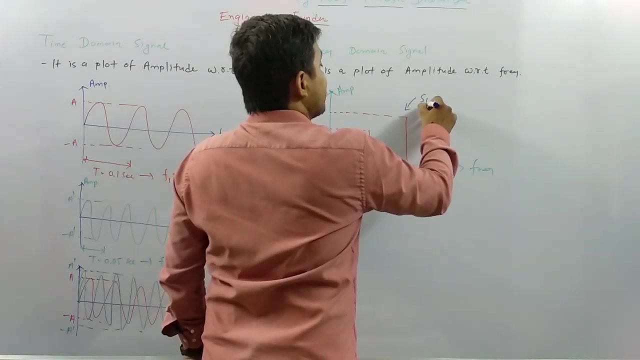 Now let us try to understand few more basics. which is there with frequency domain, Like see, when you plot that. So if you plot that combination of signals in frequency domain, that is what spectrum, which is what we are plotting. so this is referred even as spectrum. 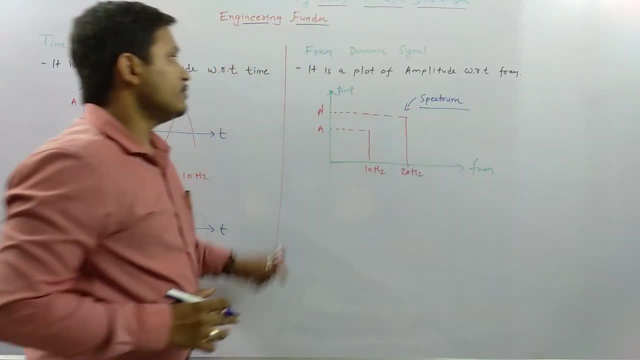 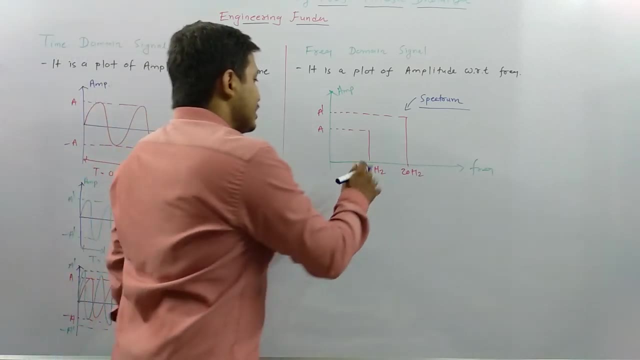 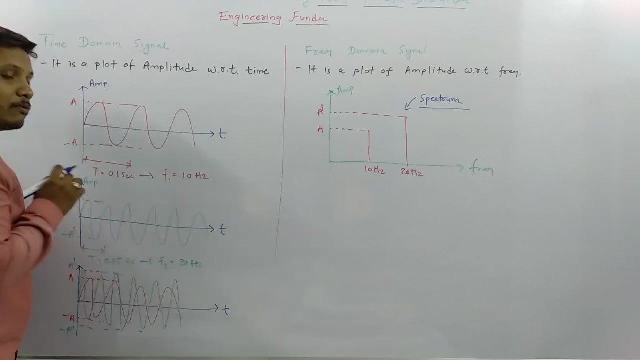 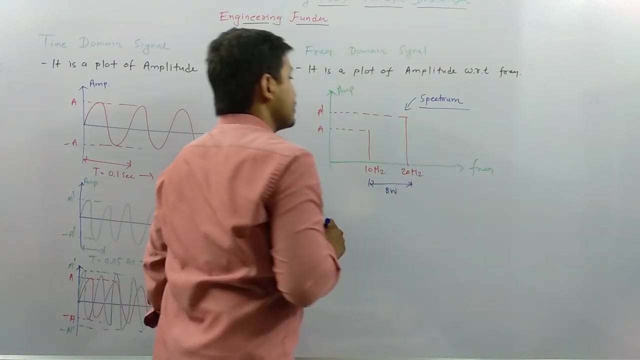 The reason is where we represent how many frequency components which is there in that resultant of signal. so that is referred as frequency spectrum And here information that is there in between this two frequencies: frequency 10 hertz and 20 hertz. so this is what my bandwidth. so this is bandwidth of this spectrum. 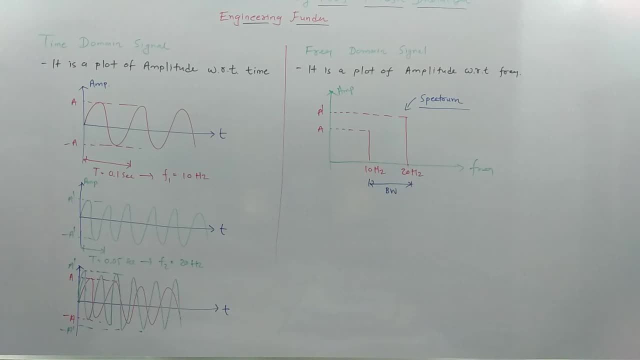 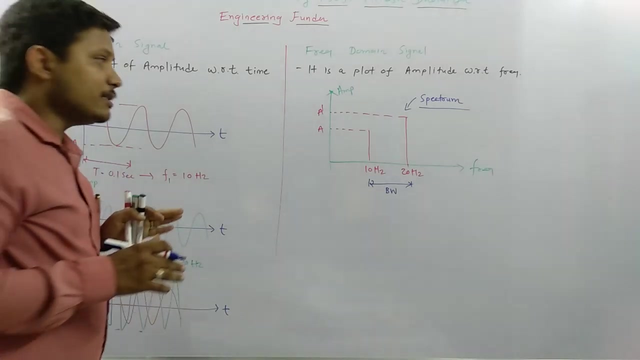 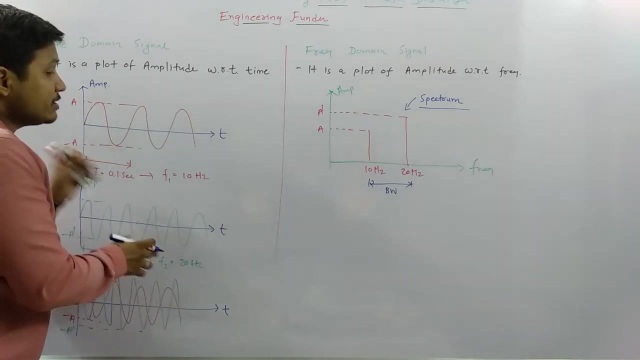 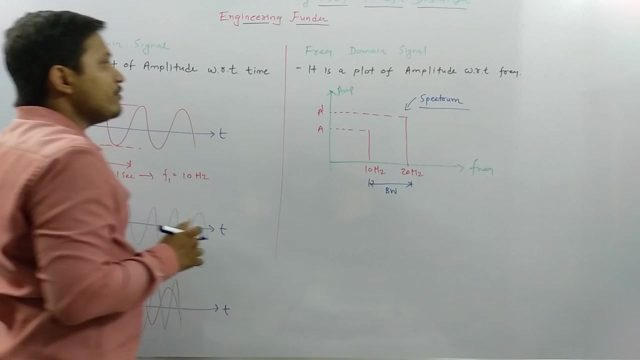 so this is bandwidth of this spectrum now when we talk about this time domain analysis of signal. so in time domain analysis of signal it is not possible to identify whether system is stable or not. but when we talk about frequency domain analysis, it is easier to identify stability. 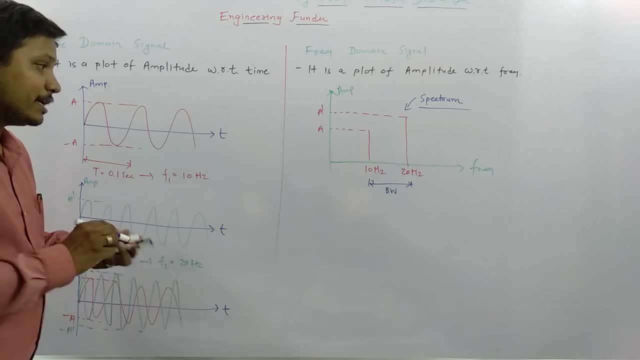 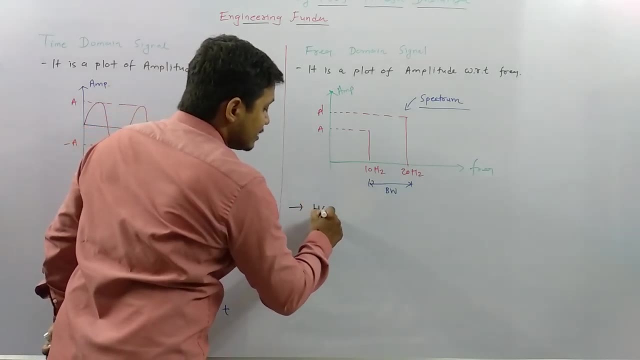 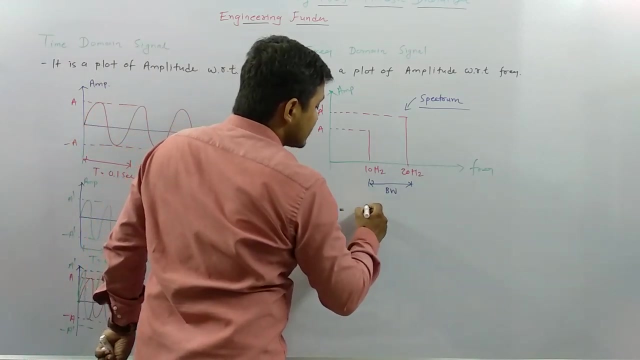 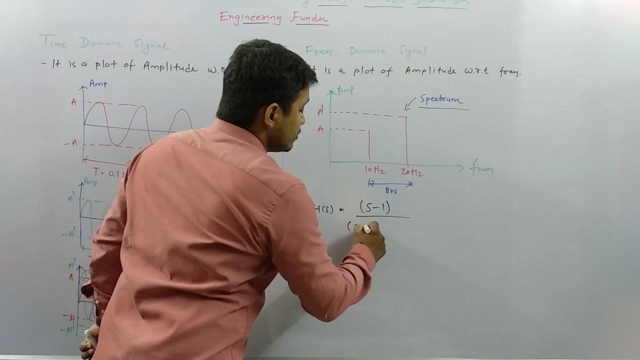 so let us try to understand how it is easier to identify stability. so, for example, if i say i have a transfer function of system, let us say transfer function of system in frequency domain, laplace domain. i am representing that as per s minus 1 divided by s minus 2. 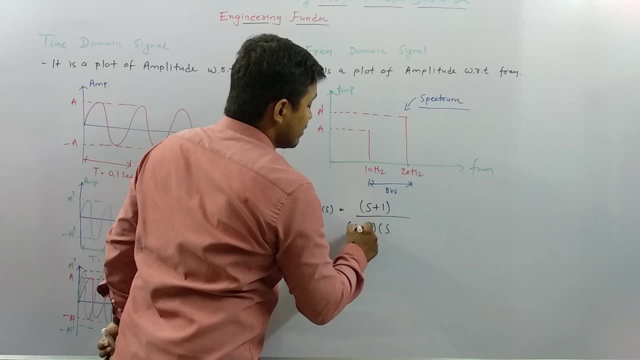 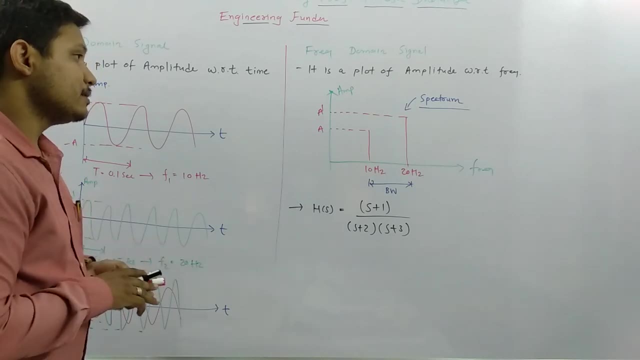 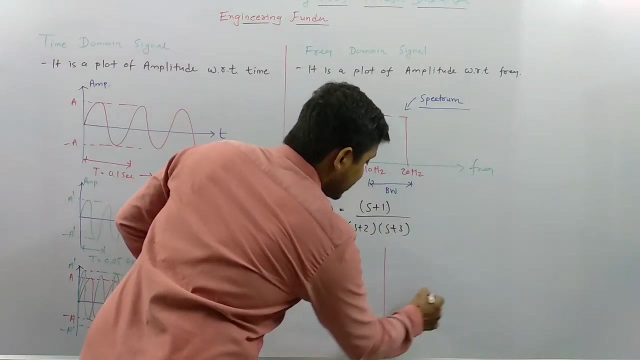 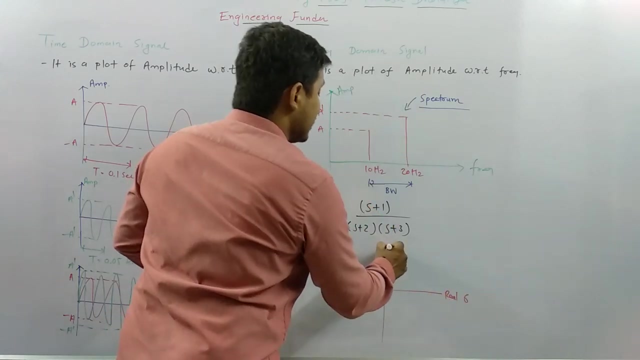 s minus, sorry, s plus 1, divided by s plus 2, s plus 3, that is how transfer function is there with this system. now, if i plot that, pole zeros. so here we will be having real axis sigma, and here we will be having imaginary axis. 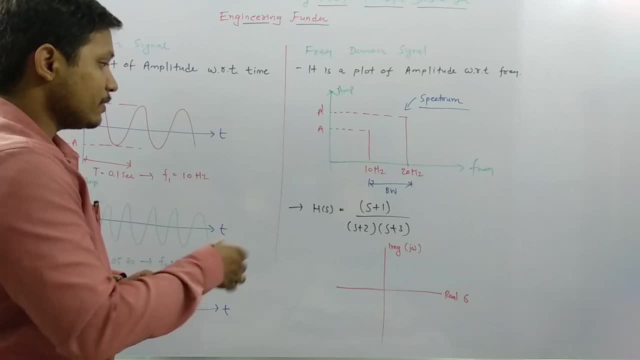 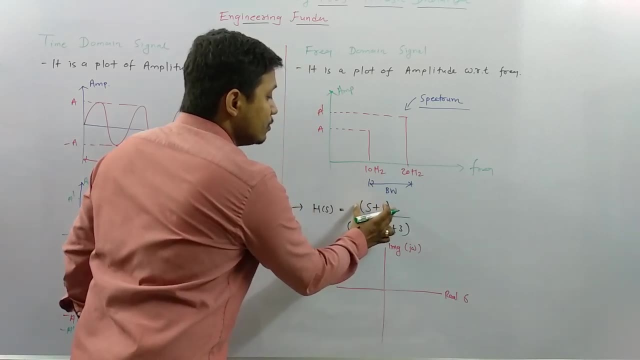 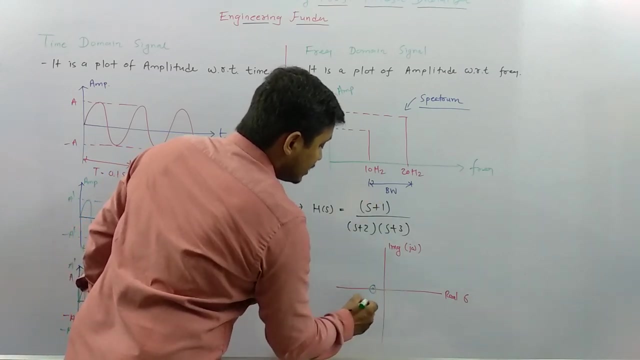 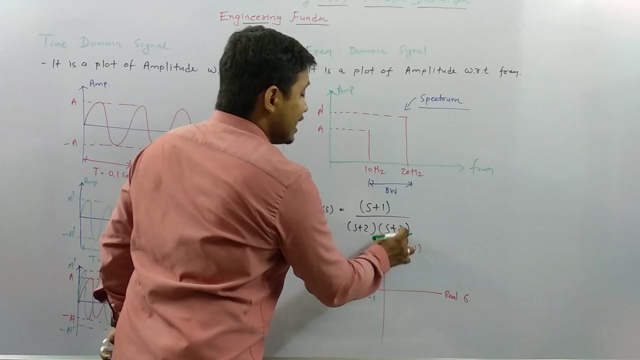 j, omega. now if i plot that pole zero, so here at s is equals to minus 1, there is zero. the reason is that root that is there in numerator, so here at s is equals to minus 1, there is zero. at s is equals to minus 2, there is pole. and as at s is equals to minus 3, there is. 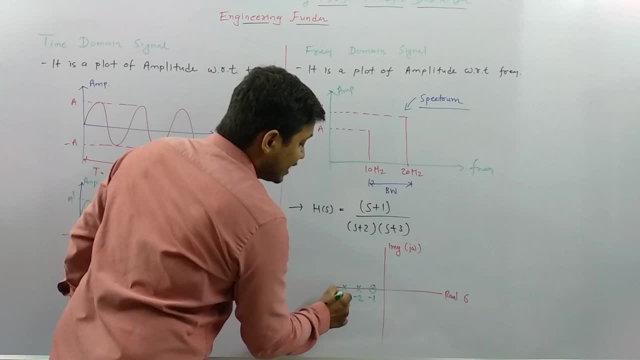 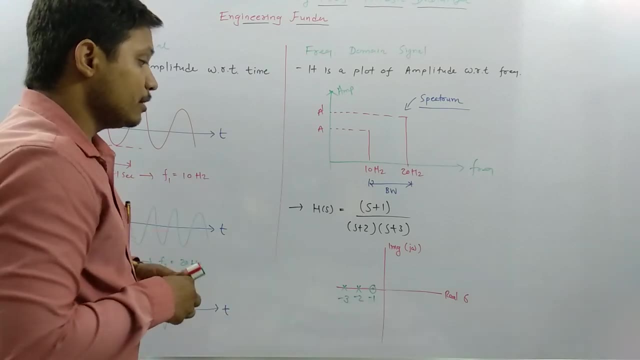 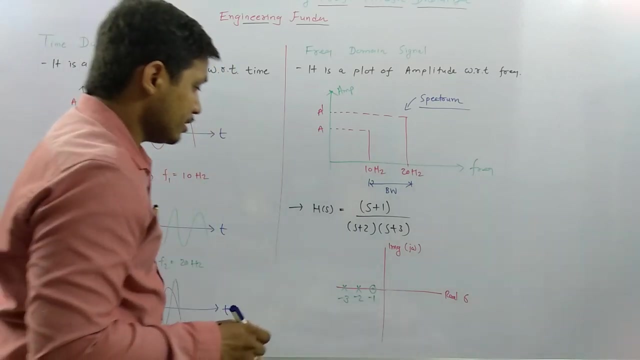 pole. so at s is equals to minus 2, there is pole, and at s is equals to minus 3, there is pole. so that is how we can analyze that on real imaginary axis or real imaginary clay. so if here, when you do this analysis with respect to frequency domain, 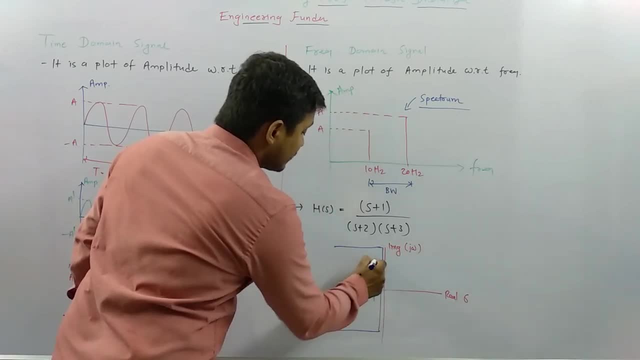 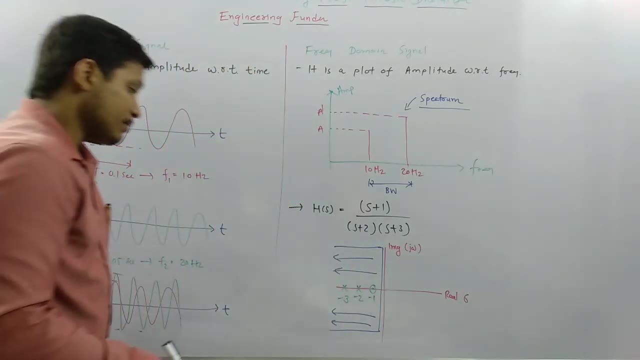 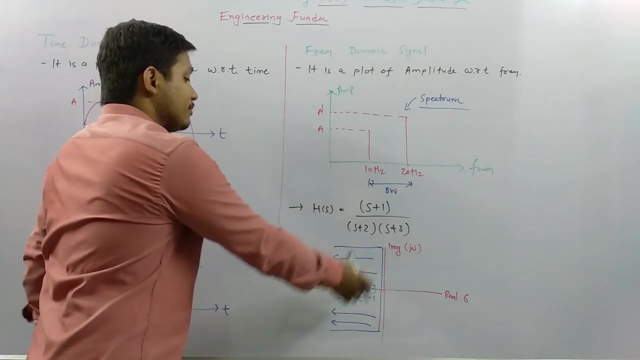 roots that is there on this left half plane. if all roots that is there in left half plane, we can say this system is stable. So if all these roots that is there in left half plane, we can say system is stable. So stability of system that we can identify. 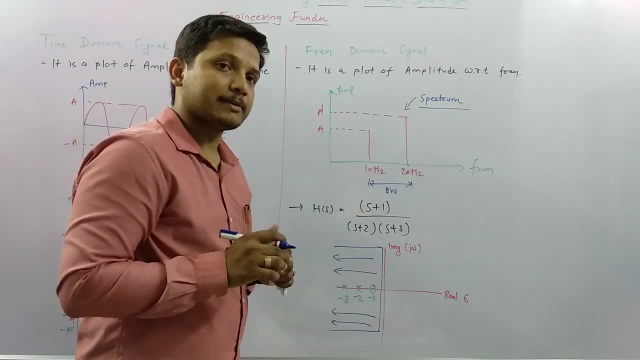 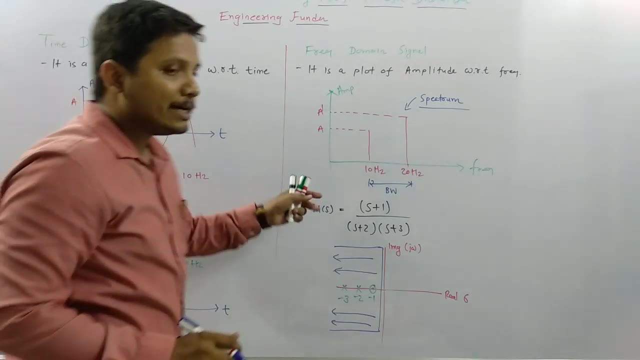 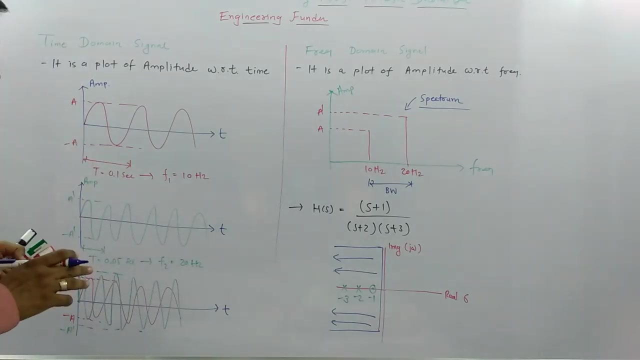 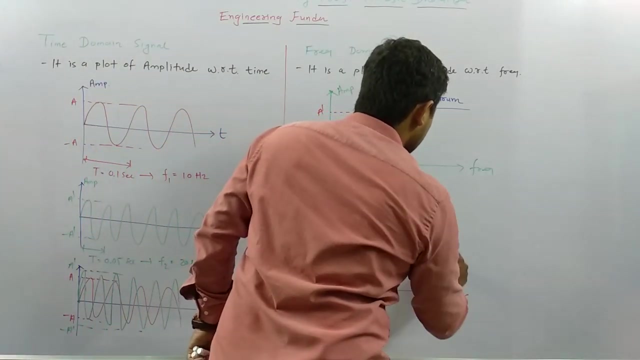 based on frequency domain analysis. So this is one advantage which is not possible in time domain. In frequency domain we can identify stability of system. So this is one advantage. Now one another advantage, that is, we can have filtering. So in filtering, what we can do is 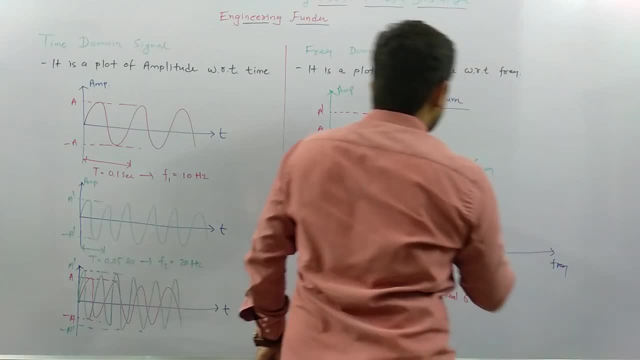 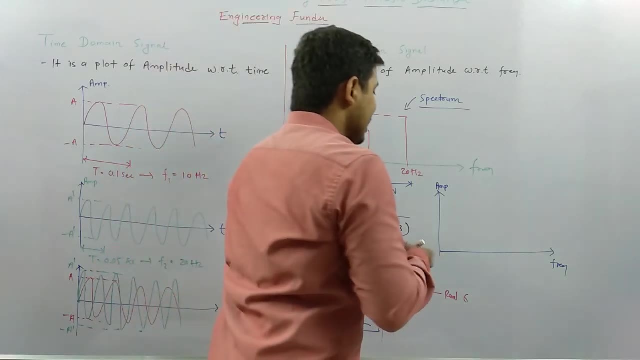 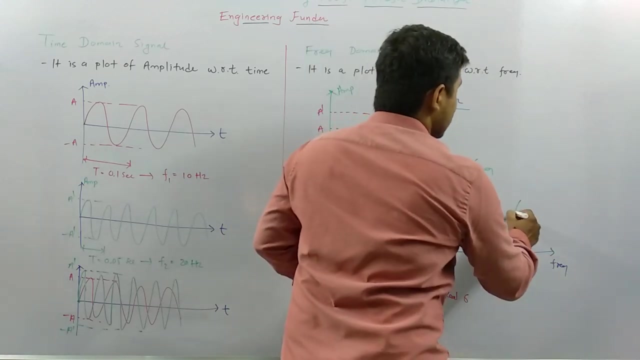 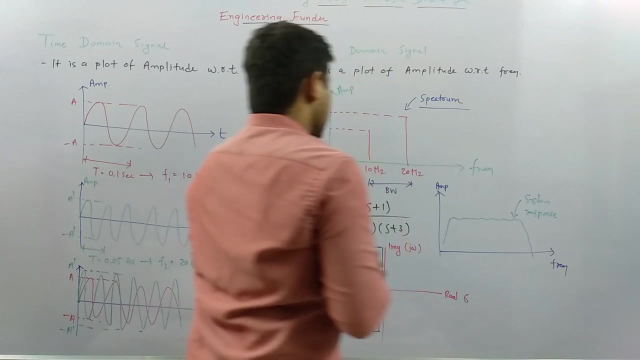 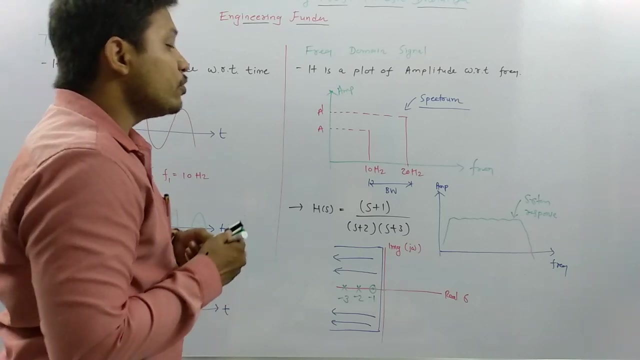 let us say this is what frequency domain, frequency response of system, where this is amplitude and this is frequency. Now, here, if I say actual system response is somewhat this: So this is system response. So this is system response right now, and now I want to do filtering operation. 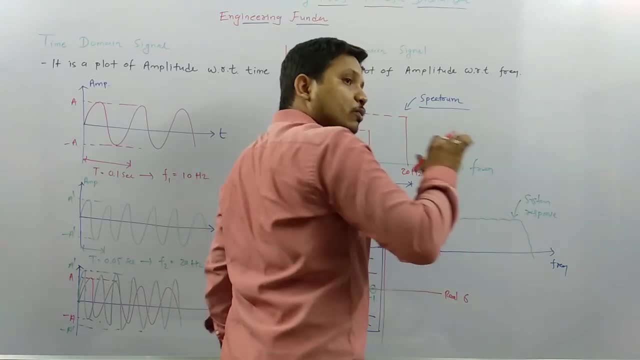 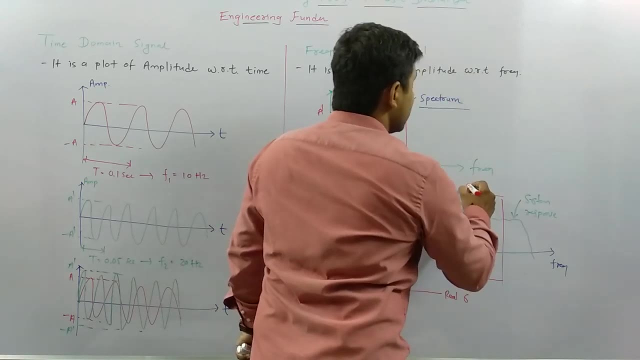 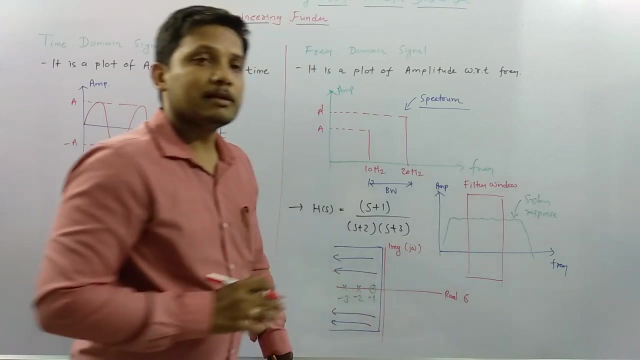 So what I will be doing is I will be passing this system through a filter. Let us say we pass it through bandpass filter. So this is my window, So this is filter window through which I am passing this response. So, after passing, 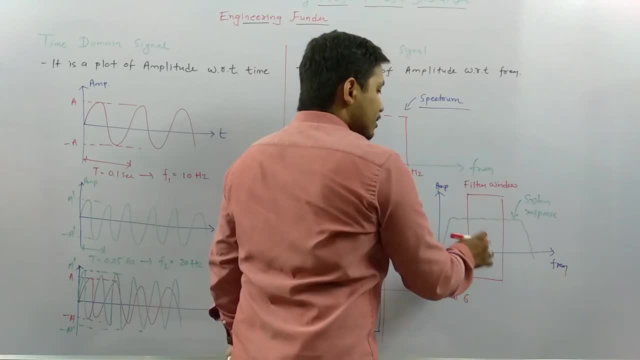 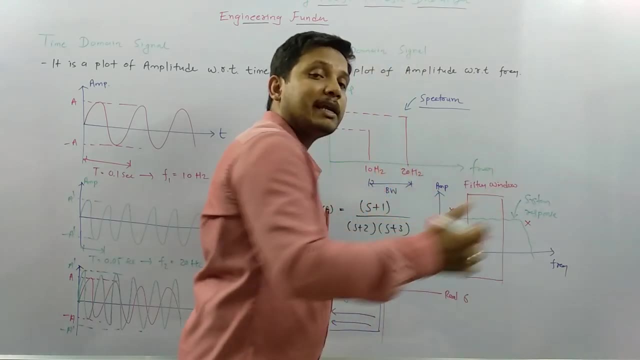 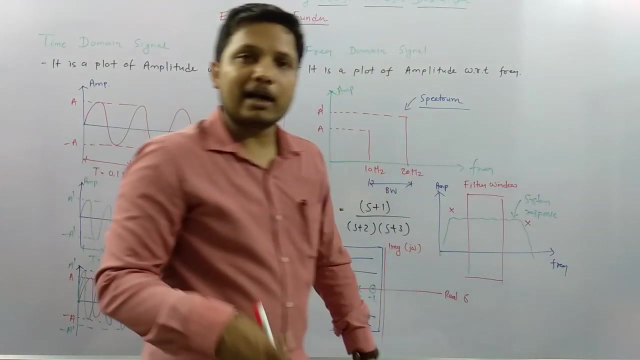 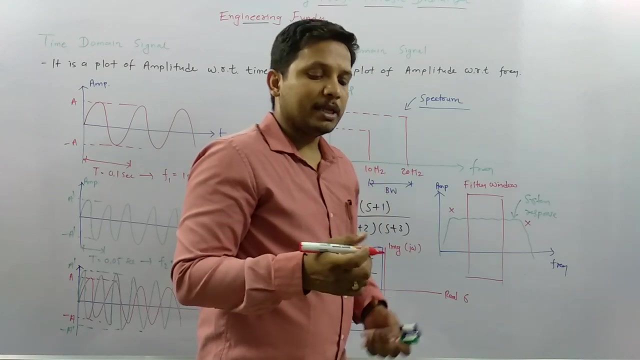 This system. through this filter, This response will get eliminated and this is what the only component which will be appearing at output side. So this components that will appear, which is there in this filter window at output side. other components will get nullified. So filtering that we can do it in frequency domain analysis. 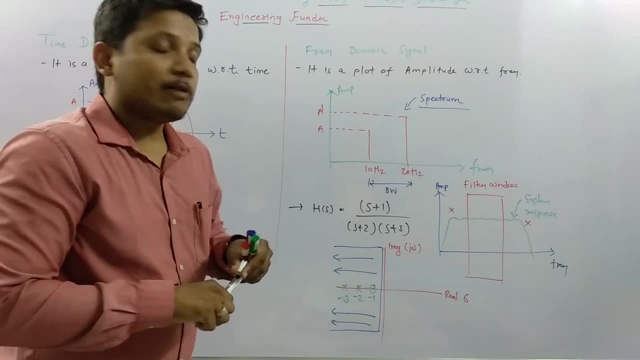 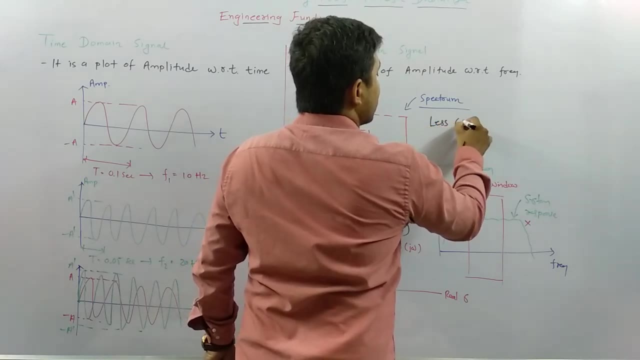 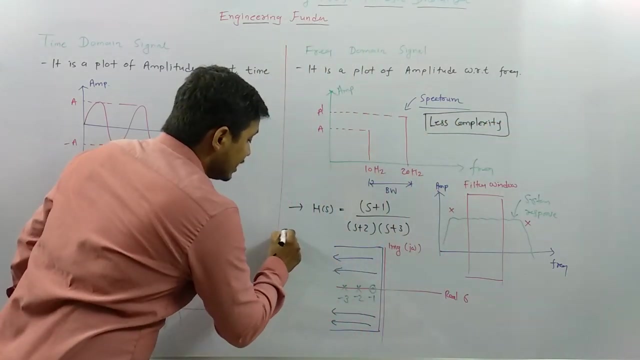 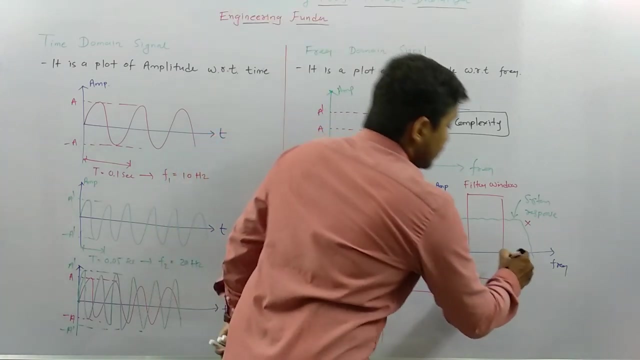 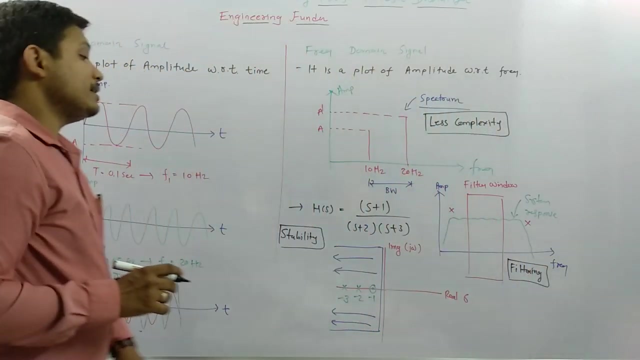 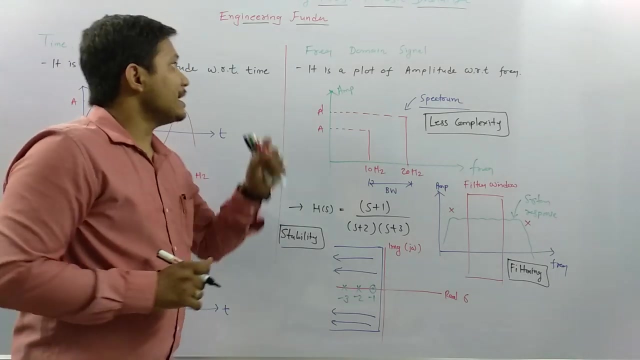 So basically three advantages That I have discussed till now: One is less complexity, Second is stability And third is filtering. So these three basic advantages, That is there, with frequency domain analysis. One more advantage is that is they frequency domain. That is like see, 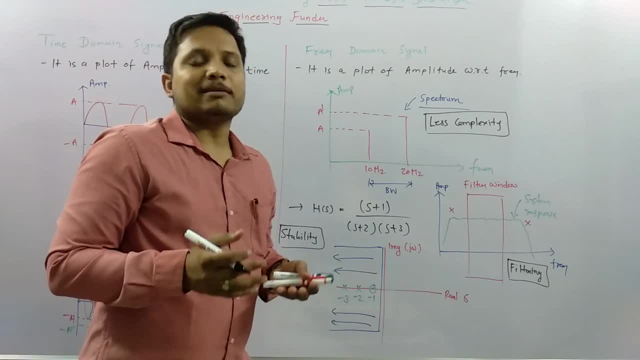 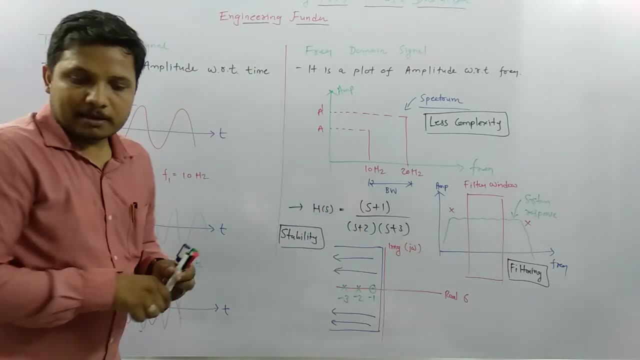 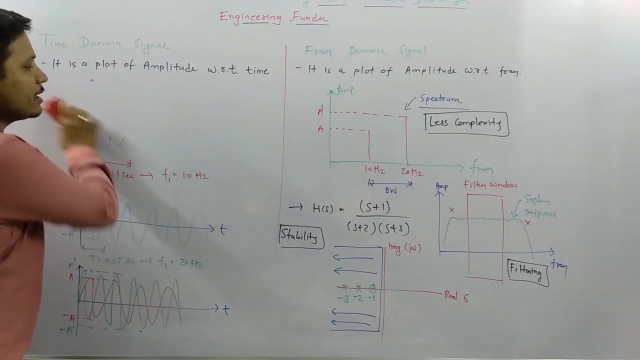 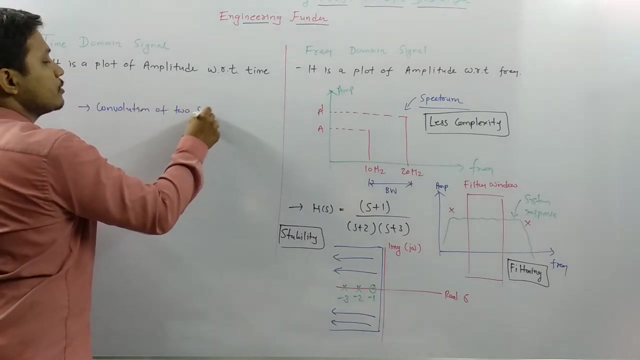 When we do, when we do convolution of two signals, That appears multiplication in frequency domain. typical expression of two signals Here of papirms: multiple efficient in frequency domain. So I am just erasing it Right now From here. Convolution of two signal appears multiplication in frequency domain. 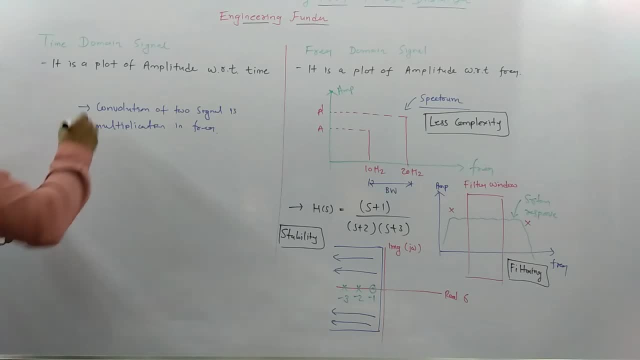 Now let us try to understand this how. this is one very important advantage. like see, for example, if I have two signals, let us say Xt and Yt, and if I do convolution of this, then that will result into response. it could be somewhat response now if you do that in frequency. 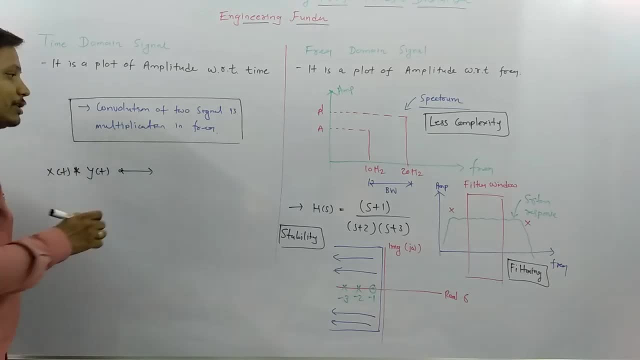 domain, then that will be just a multiplication. you do need to do convolution. So this is the symbol of convolution now in frequency domain. if I say Xt represented by Xf and Yt represented by Yf, then that is just a multiplication in frequency domain. 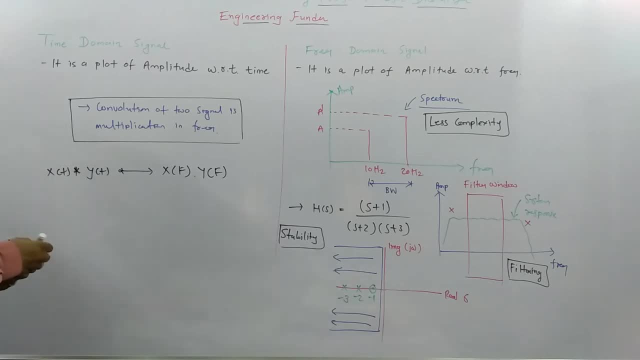 Now to get response in frequency domain from time domain, all we need to do is you can have Laplace transform, you can have Fourier transform Or you can have Z transform, and Z transform could be done in case of signal is discrete signal. we can have Z transform to have frequency domain signal. 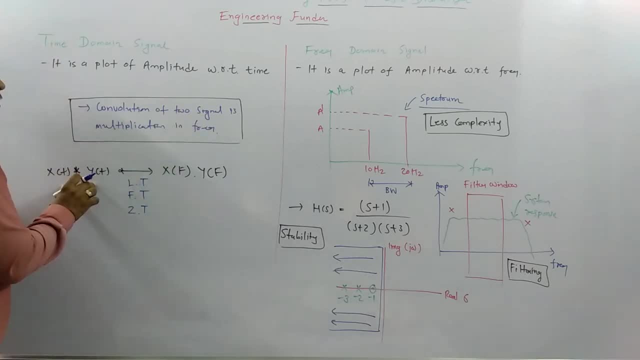 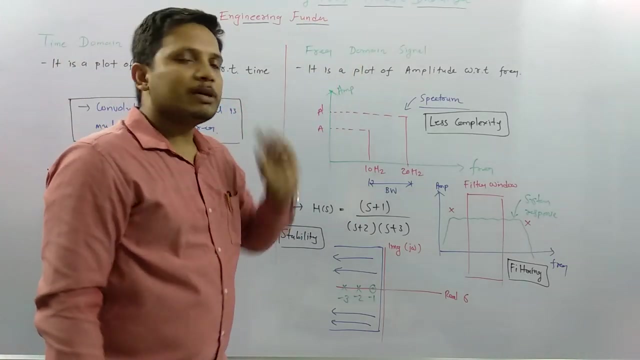 So convolution of two signals in time domain is multiplication in frequency domain. so that is even one very important advantage that is there with frequency domain analysis. So basically there are four major advantages which is there with frequency domain analysis. One is frequency domain analysis compared to time domain analysis. one is less complexity. 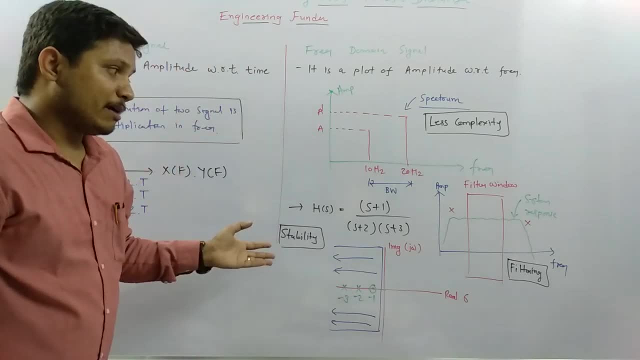 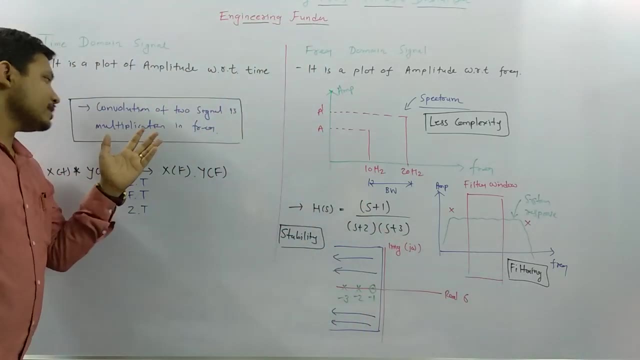 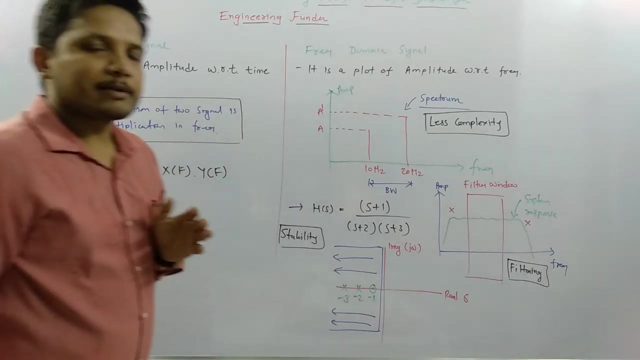 in representation. second is identification of stability. third is filtering could be done in frequency domain analysis. and fourth is convolution of two signals is multiplication in frequency domain. Now there are few disadvantages or drawbacks. that is there with frequency domain. one is we cannot identify phase of signal. 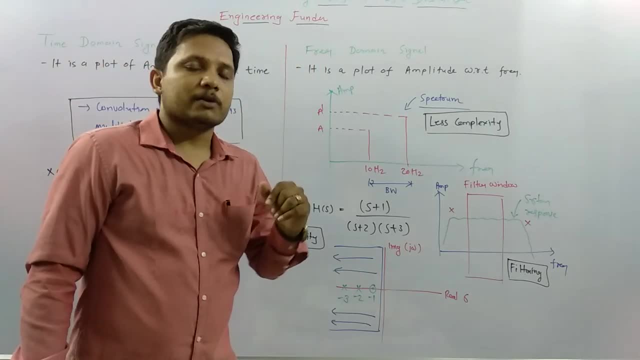 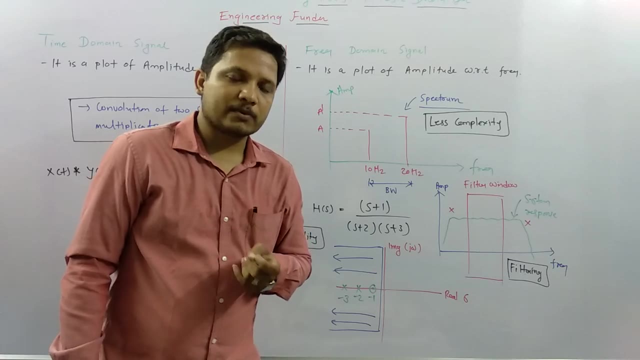 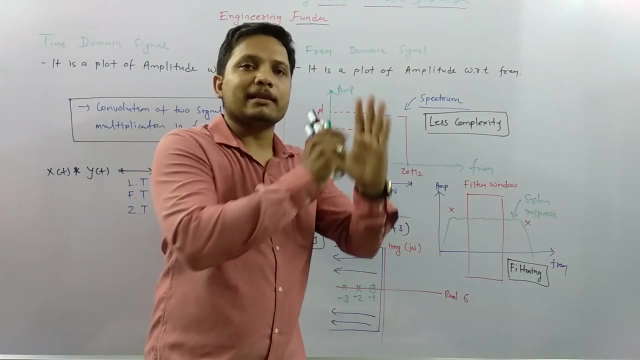 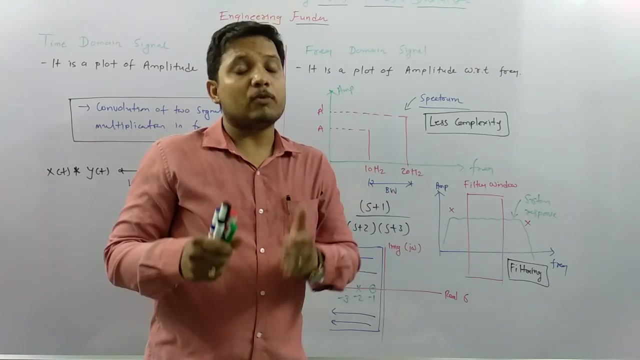 By frequency domain analysis, so phase of the signal could not be identified by frequency domain analysis. and one more disadvantage. that is like when we transmit signal which is analog one, before we transmit that we convert that into digital one. Now, to convert that into digital signal, we do quantization. 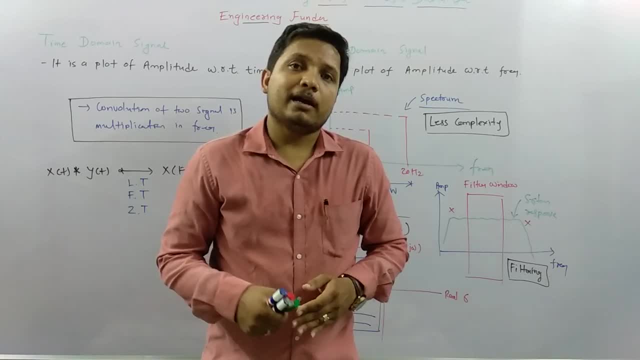 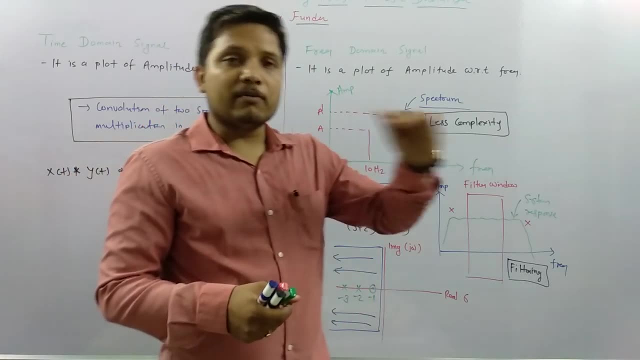 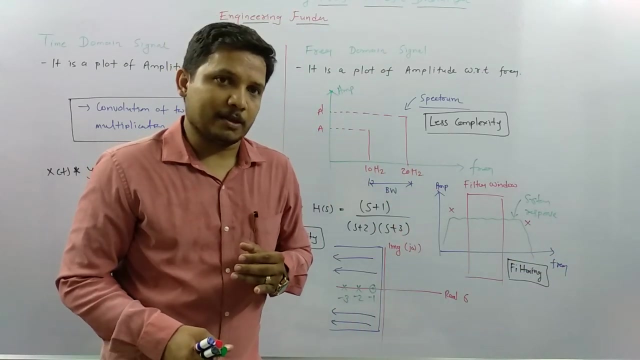 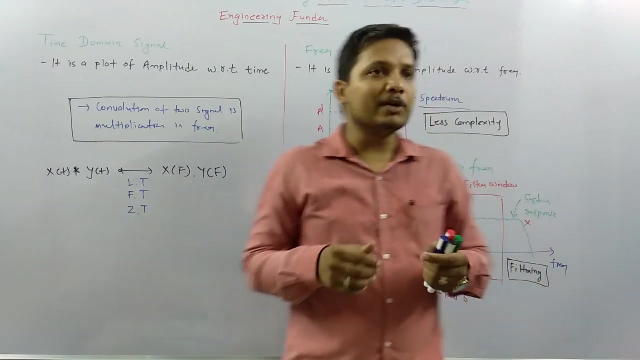 And in quantization, everything is there in terms of time domain. And after translating that signal in digital domain again, we send it over some frequency and we receive that. and after reception, every process that we do it in terms of time domain. So that analysis, that understanding, that requires time domain analysis where you cannot utilize